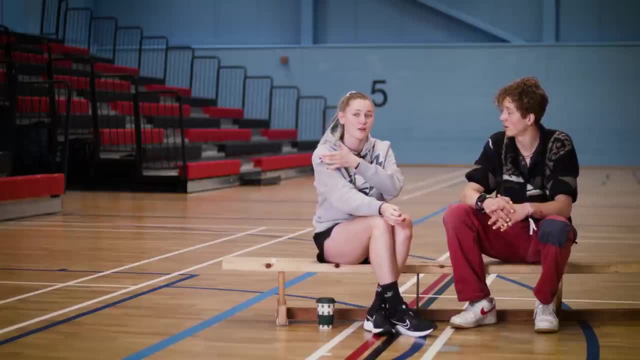 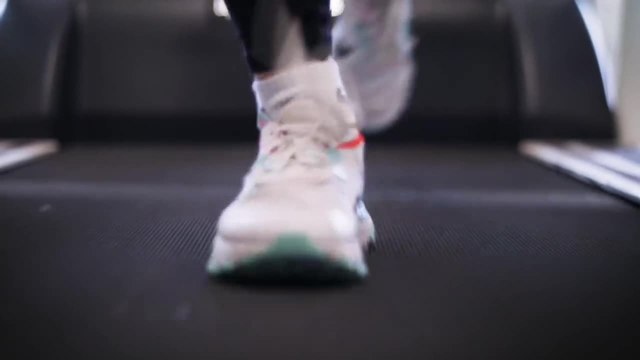 or helping just the general public be healthier. So you do learn a lot about people and how they work. If you're doing an examination of someone like a fitness test, of someone like running their CPET exam, they're going to be very anxious, like you know. 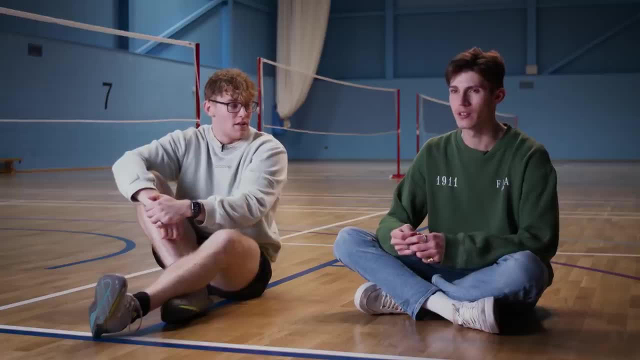 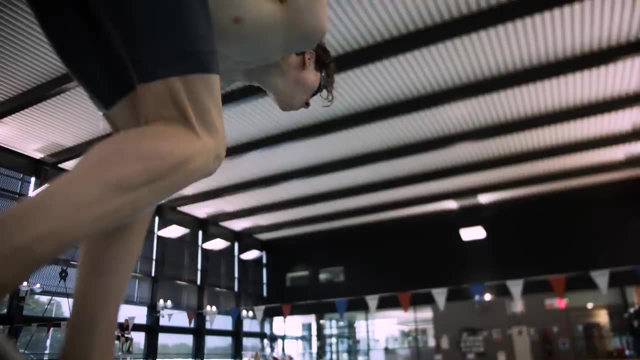 is there something wrong with me? So there's quite a lot of focus on people in that respect. It's not only how they work, but how to treat them in like a professional sort of context. We'd be learning a lot more about people. 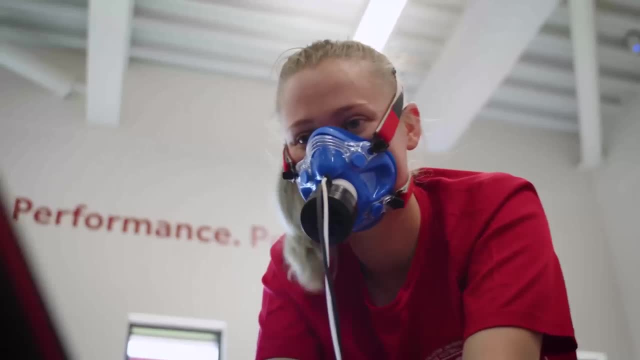 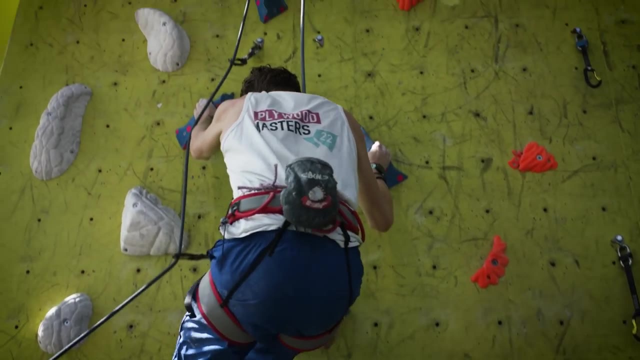 and learning about. like cold water swimming. in psychology They take us cold water swimming. We were learning about scuba diving and physiology. We go scuba diving. We went scuba diving. We go back home, like to all the people not doing sports science. 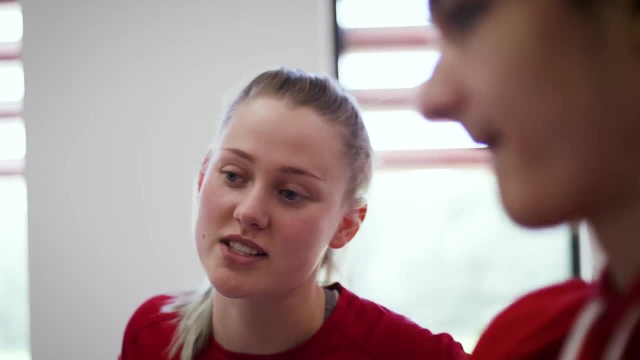 and like: oh, what are you doing this week? Oh, we're scuba diving. Yeah, Oh, what are you doing this week? There's just so many doors, doors that are open. I know, I think, the people who are in your year, 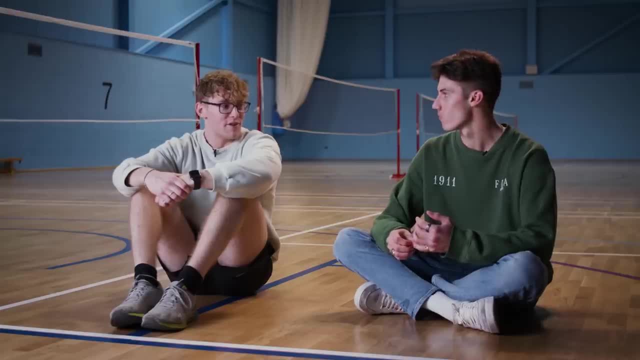 that have. I think they've started up their own sort of businesses, But then you learn how that some people on the course are actually going to be doctors. Yeah, exactly, And that's what they're going to do. Like you could be sat in an interview for a job. 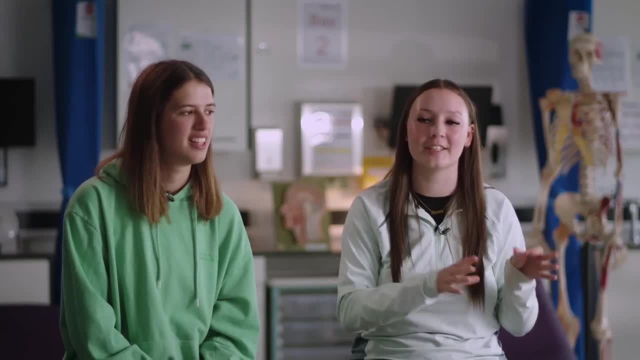 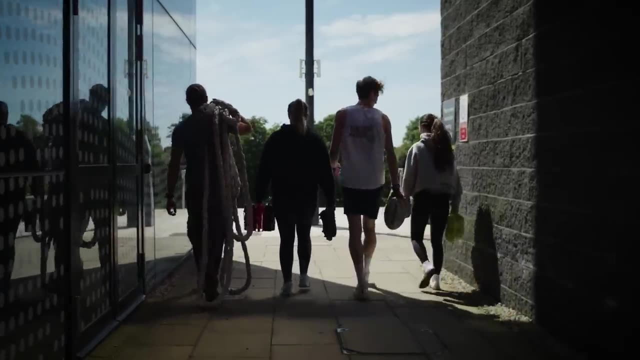 and they'll say: tell me your time, you've done this. and they have literally set us up to have done. like every single- Yeah, they've hit every single one, like every single skill, every single opportunity, Like they've set us up, like essentially. 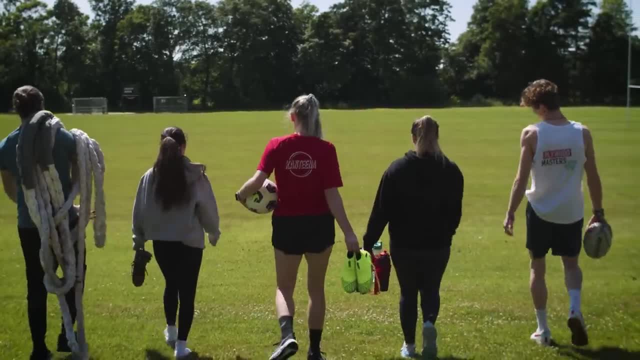 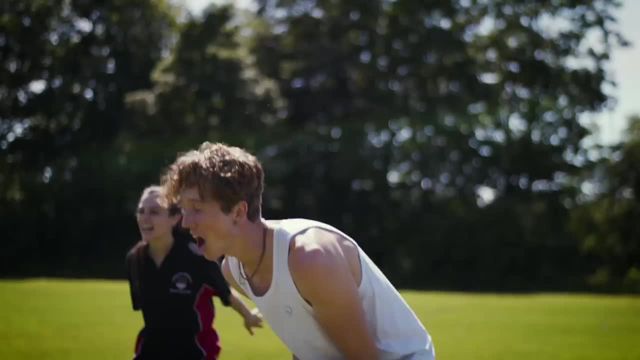 Very active people generally. There's all kinds of people on the course and it's like. I quite like that as well, because it means you meet just loads of different people at loads of different ages as well, which I was quite surprised at. 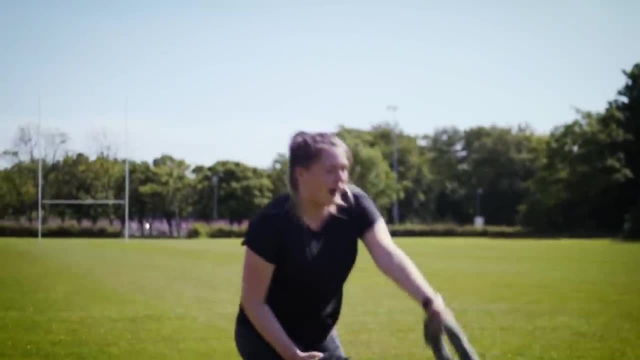 I think like competitive nature is very, very obvious. Yeah, Oh God, yeah, definitely Like when you've been brought up in sports for 21 years. Yeah, you need a bit of oomph. Yeah, exactly. 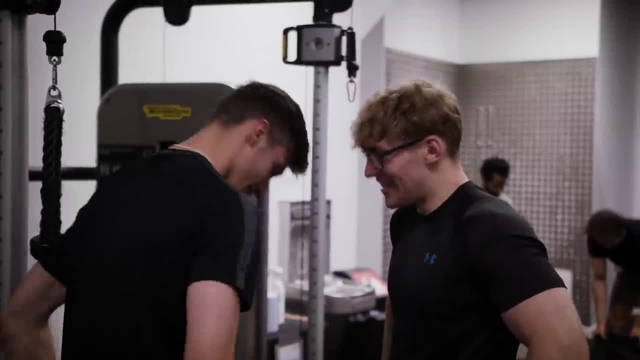 You know straight away you've got something to talk about with everyone. It's like the icebreaker, isn't it? Yeah, it literally is: What sport do you play? What sport do you play? Who do you support? When do you play? 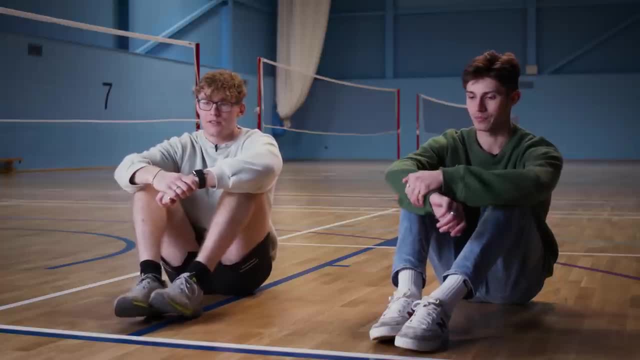 Yeah, So we can come watch you, Because that was something that we did in first year. quite a lot was we'd always go and watch each other's games, Even like the lecturers. how well the lecturers are involved with us. 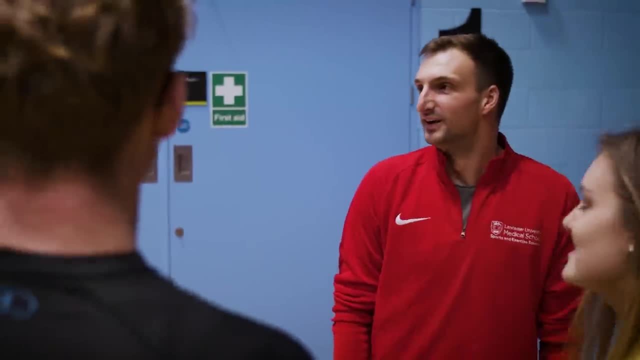 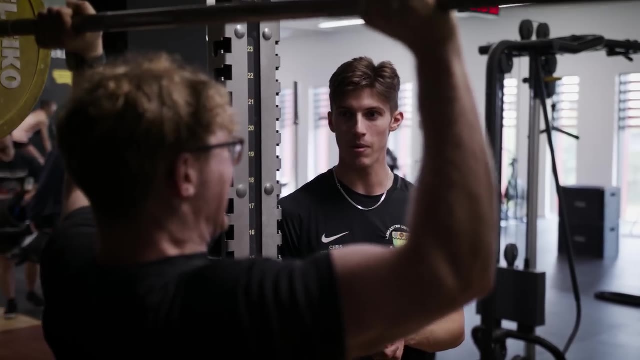 and they're so like enthusiastic for us to be like this big group of friends. basically, You were about to be cheesy and say family then, weren't you? Yeah, I think they like put us into situations that at the time,